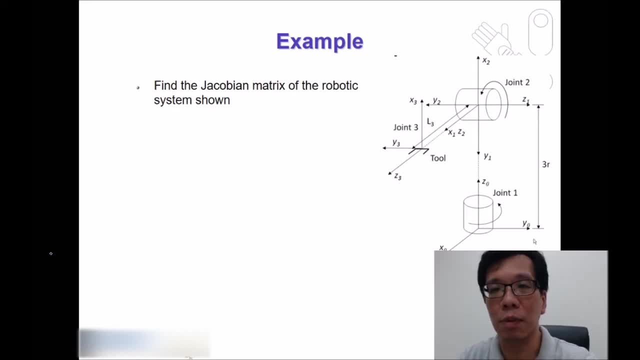 little bit about what's going on. So if we want to find out the transformation metrics, the first thing we would need to do is to set up the table, just like what we did many times. In this time. we have link 1,, 2, and 3, since we have three. 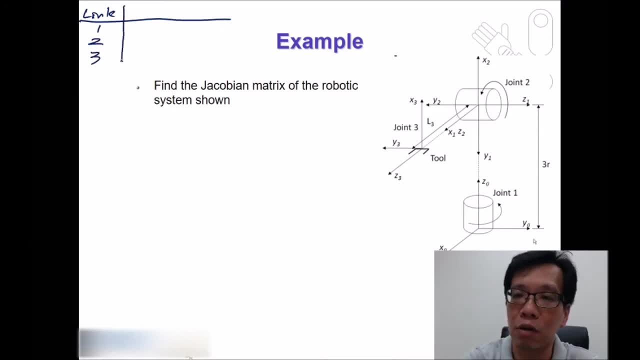 joints. So we're going to have something like this and we're going to have the corresponding coefficients, ai, alpha i, di and theta i. Clearly, the first one is a revolute joint, So we have theta 1 over here and the distance between the first joint and the second. 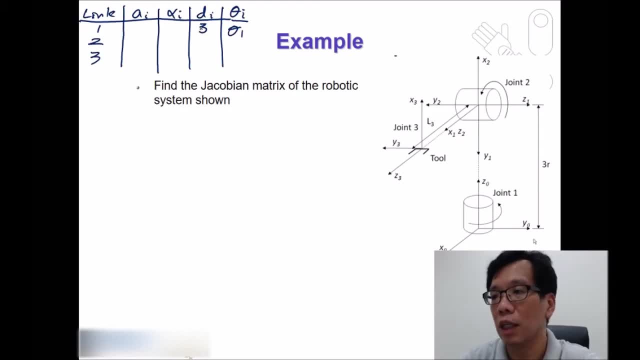 joint is 3 meters, So we mark as 3 over here. This one, z1, is in this direction and z0 is in this direction. So in other words, the rotation is along this direction, which is going to be negative pi over 2. And a over here. 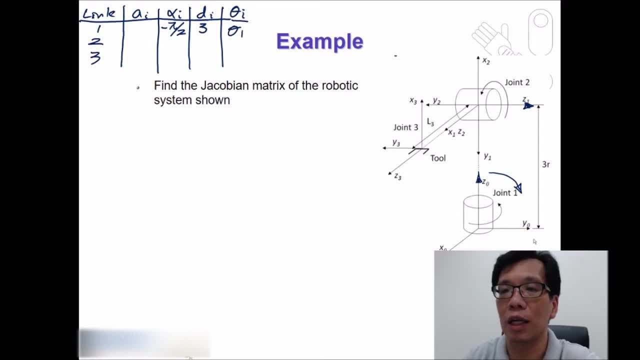 since we do not have any movement along x axis. so this one over here is going to be 0.. That's the first one, So we have the number we have in this table For joint 2, this one is also rotational. So we have theta 2 over here, and this time the tool n has not. 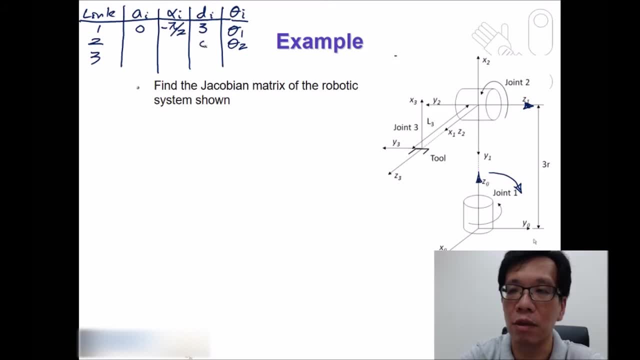 moved along z direction, So this one is going to be 0.. Over here, z has been changed its direction from this one to this one. Let's see another negative 2 pi over here, So just mark it as this one. over here again. Again, we do not have any movement along x direction in this. 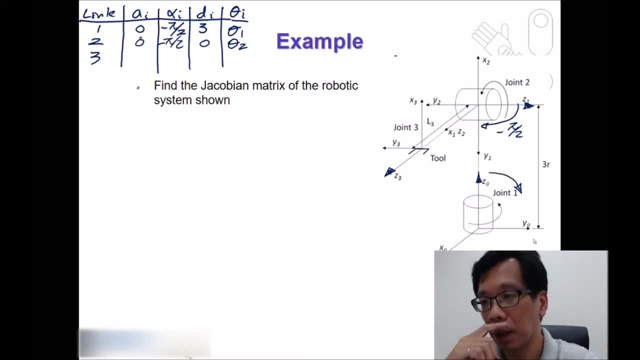 direction. So it's going to be 0 as well For the first one, since we do not have any revolute joint over here. So theta in this case is going to be 0.. And this one is moving along the axis which is L3.. 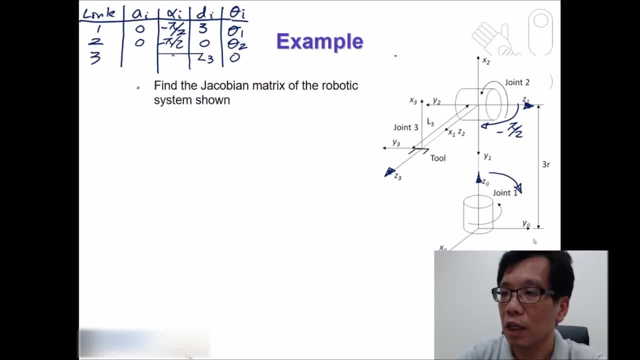 So we mark L3 over here. We have the same coordinate over here, So the alpha is going to be 0. And A is going to be 0 as well. So this completes our table of coefficients. Now we would need to find out what's going on. 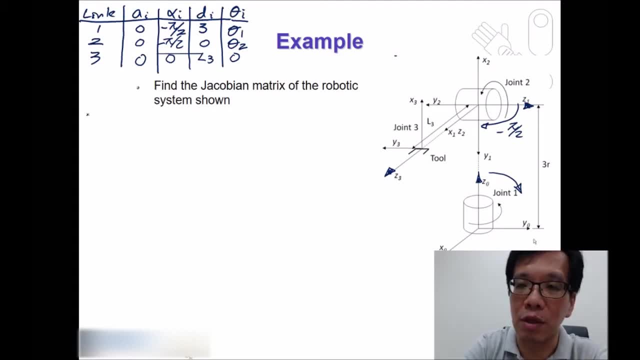 For the transformation matrix Now, since we're doing Jacobian, so there is something we want to do in the first place. We talk about A0.. A0 means that I'm rotating and translating myself into myself, Which means I'm not moving anywhere. 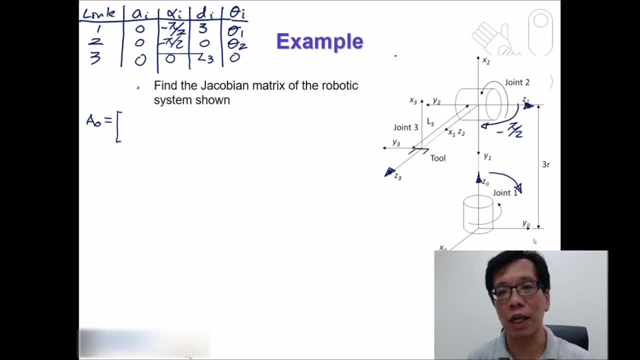 And all the angles are equal to 0 degrees. So with that said, A0 over here is actually Sorry, I'll erase this one Identity for the rotational part And for the translational part it's going to be 0.. 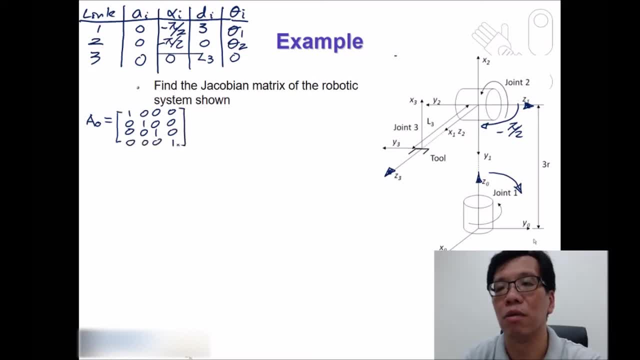 The fourth row over here is also housekeeping stuff: 0,, 0,, 0, and 1.. That is my A0.. If I want to do A1 from 0's frame to the first frame, it is also 0 to 1.. 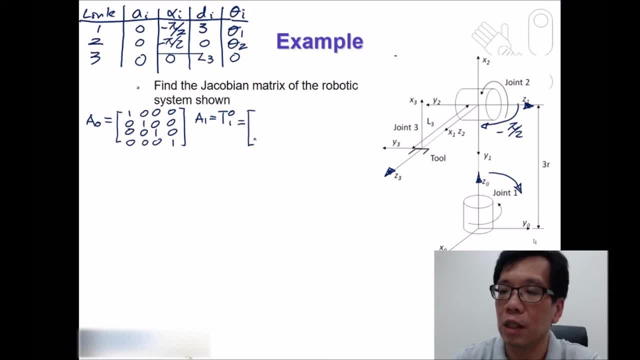 So when we do this, this one over here, please be sure you're going to follow a specific formula that we have been talking about many times, That is, The translation matrix is going to be rotational about theta And translational about d. 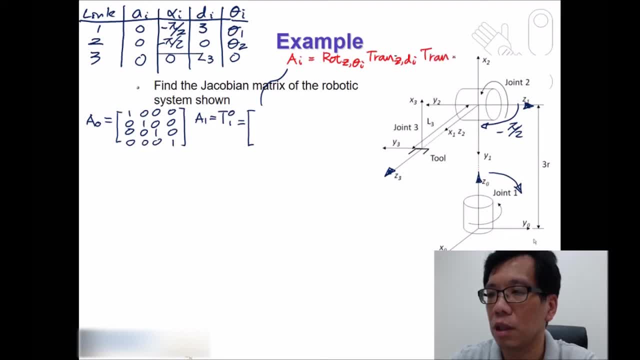 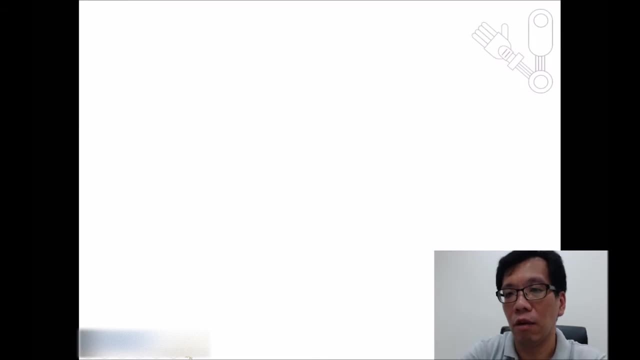 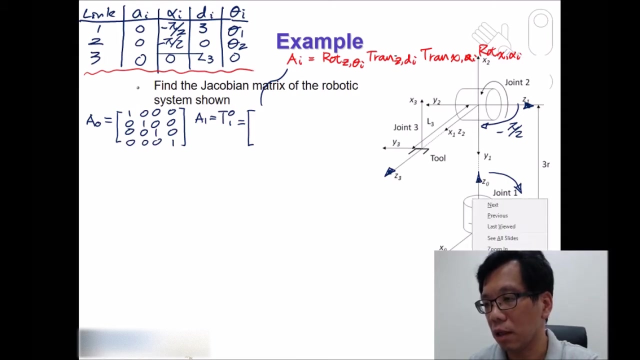 Translation matrix x about ai- rotational x direction- with alpha i. So this is going to be the matrix that we're going to deal with for all the four coefficients over here. So that's it. Let's write down the components based on the configuration we have. 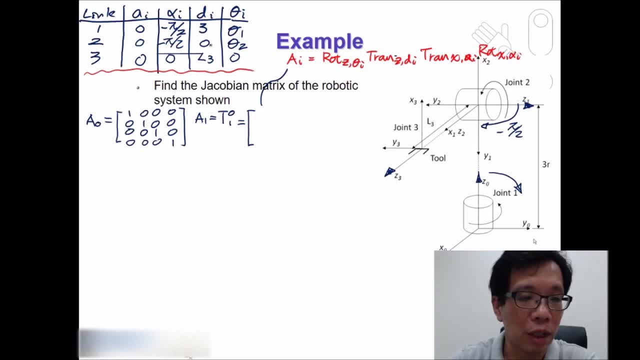 So over here. if you follow the table over here, you should have cosine theta 1, sine theta 1, 0, 0, minus 1, 0, and negative sine theta 1, cosine theta 1, and 0. 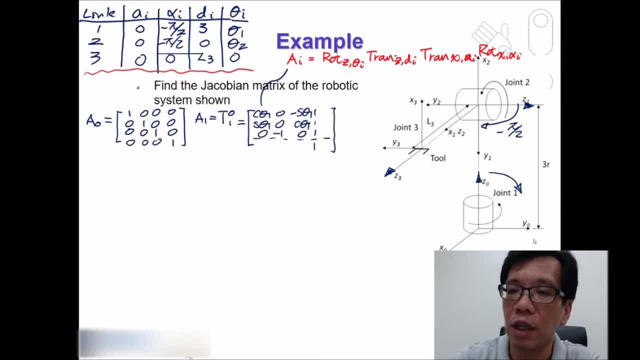 Over here we do have a translation along the S's, so it's going to be something like this: Last row, it's going to be something like this: So that is going to be my A1, and it's also my transformation matrix from 0's frame to the first frame. 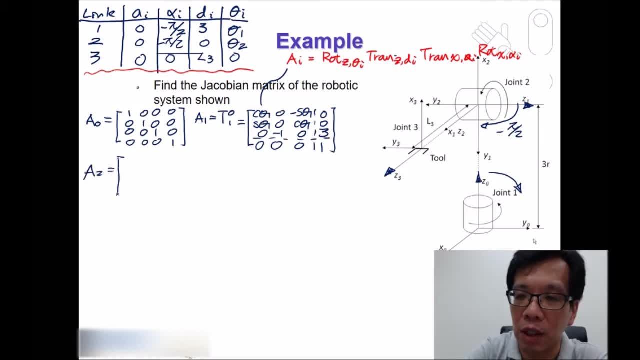 For A2,. essentially it's going to be the same thing as A1, but we have cosine theta 2, we state: sine theta 2, 0, 0, 0, negative 1, negative sine theta 2, cosine theta 2, 0.. 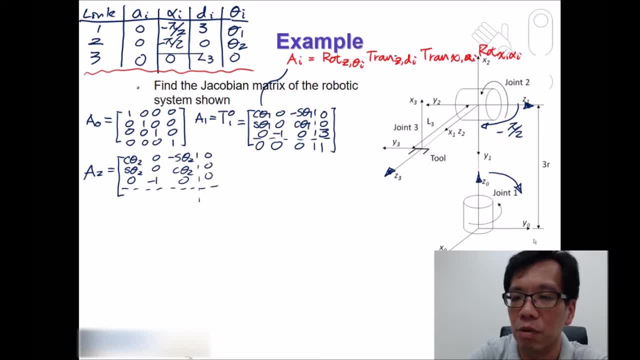 We do not have any linear moment, so just put three 0's over here and everything is going to be 0 over here. That is going to be my A2.. For A3, all the angles are 0, which means in the rotational part. 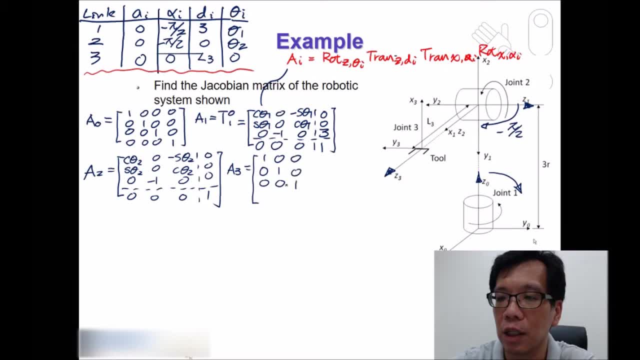 it is going to be identity, But for the translational part, I do have L3 over here, So keep in mind you will need to put your L3 as this component over here. So this one, those four matrices, are going to be my translation. 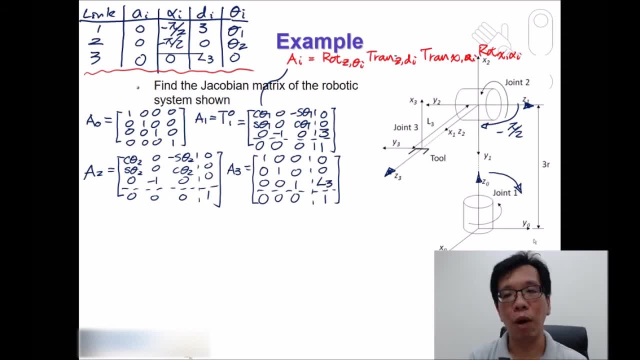 from one frame to another. Now what we need to do is to find out all the transformations from 0 to second frame, from 0 to the third frame. That should be pretty straightforward. This one over here is going to be A1,, A2, or. 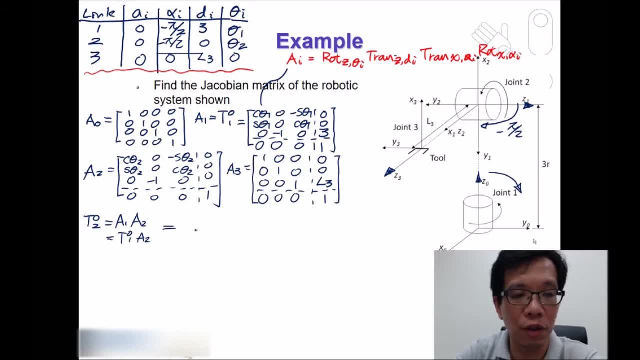 they are actually identical. So if we do something like this, we are having cosine theta 1, cosine theta 2, sine theta 1, cosine theta 2, negative sine theta 2, sine theta 1, negative cosine theta 1,. 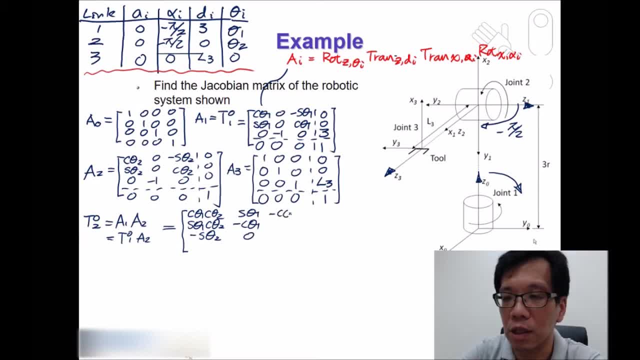 0, negative cosine theta 1, sine theta 2, negative sine theta 1, sine theta 2, negative cosine theta 2, and the translational part is going to be something like this: Then we fill the last row over here. 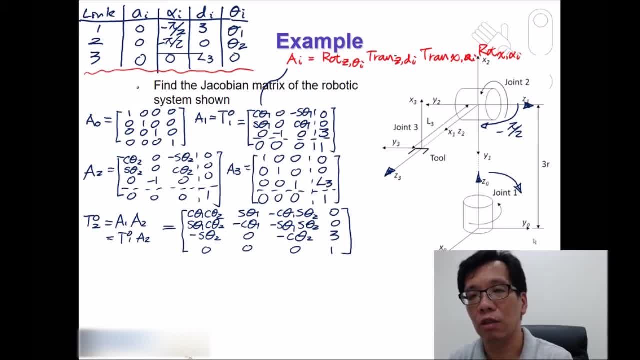 We do not only need to find out the individual transformation matrix from one frame to the other, we also need to find out the transformation from 0's frame to all the individual frames. So that's the reason we have t from 0 to 2.. 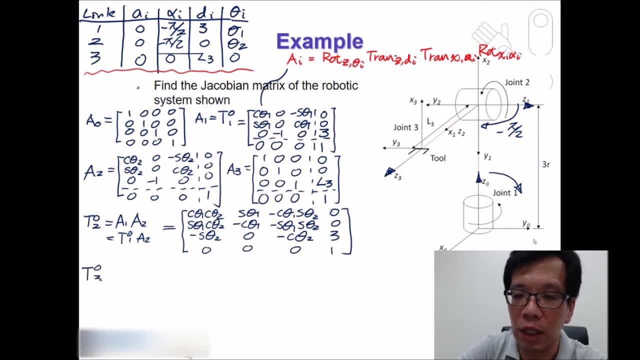 We also need to have t from 0 to 3. In this case, we are having A1, A2, A3. Or we actually have 0 to 2 multiplied by A3. Those two are actually identical. What's good is A3 is actually. 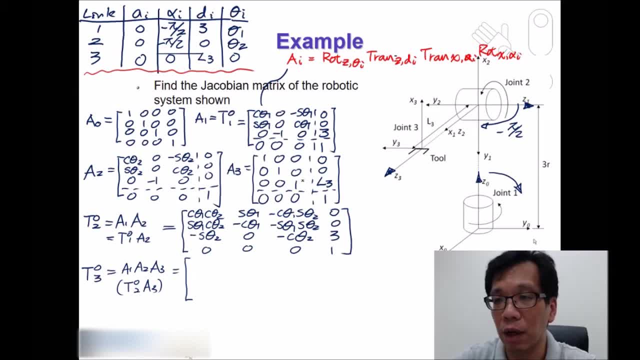 identity for the rotational part over here. So the first nine components are actually identical. We can just copy those things from this matrix to this matrix. We do not need to do any calculation again. But this one over here because of the calculation. 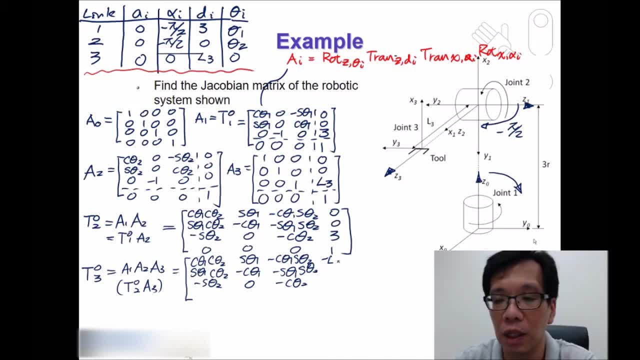 is going to be a little bit different. It's going to be negative: L3 cosine theta 1, sine theta 2.. Second component: over here is going to be negative: L3 sine theta 1, sine theta 2.. Third component: over here: 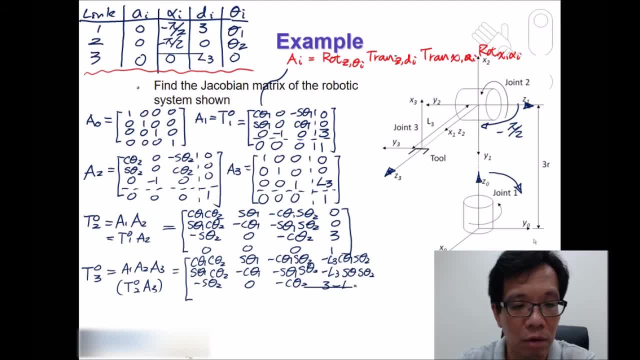 is going to be 3 minus L3, cosine theta 2.. Then the rest is going to be similar. Keep in mind there are a few components we would need to use over here. So before we start, move to the Jacobian derivation on the other side. 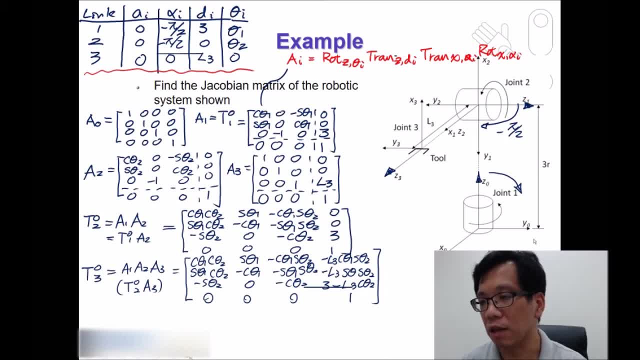 There's more of those things, So it's easier for us to find out what we need to use later. So there are two kinds of information we would need to have over here. The first one is Z naught, Z naught, and Z1 and Z2.. 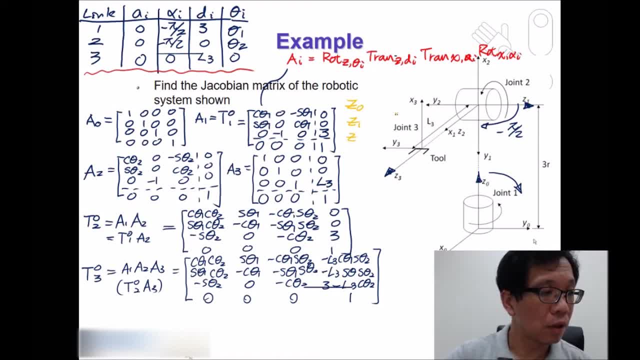 So we would need to have this one. We also need to have this one, And we do not need to have this one because it's a translation from one to the other. We always need to have the translation or transformation from zero to individual ones. 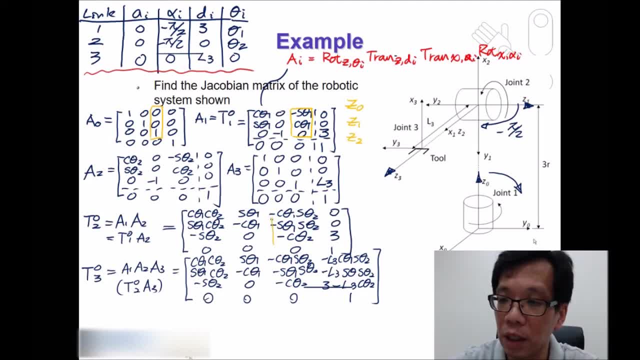 So this one over here is going to be this one That's Z2.. That's Z1.. This is zero, naught, This is Z2.. And also, we would need to find out what is my frame So over here. 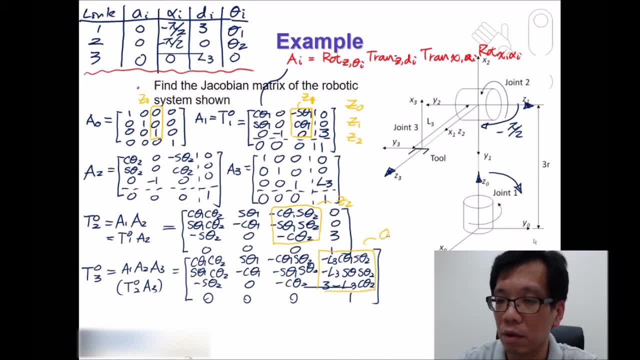 this is O3. And this is going to be O. naught, This is going to be O1. And this is going to be O2. O1. And this is going to be O2. O2., O2., O2.. 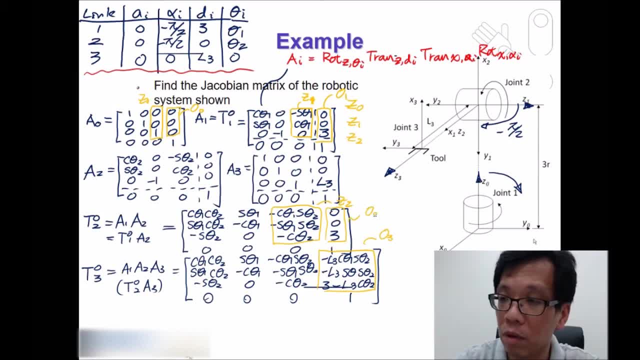 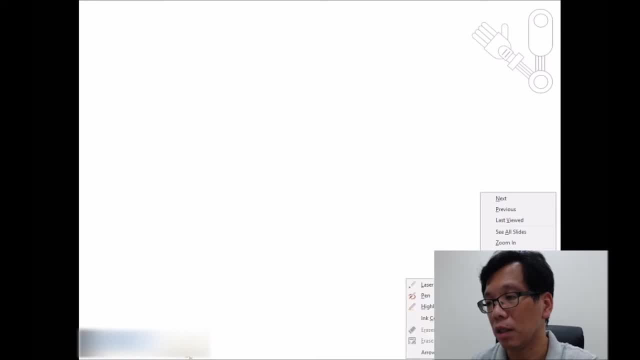 O2.. O2.. Okay, So we marked everything down. Then let's start to do the Jacobian derivation. Okay, So we marked everything down. Then let's start to do the Jacobian derivation. So let's go back again. 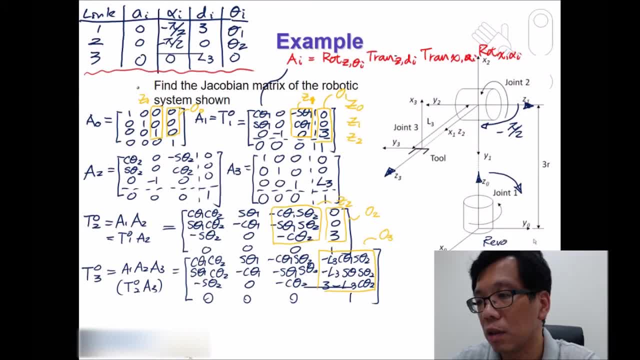 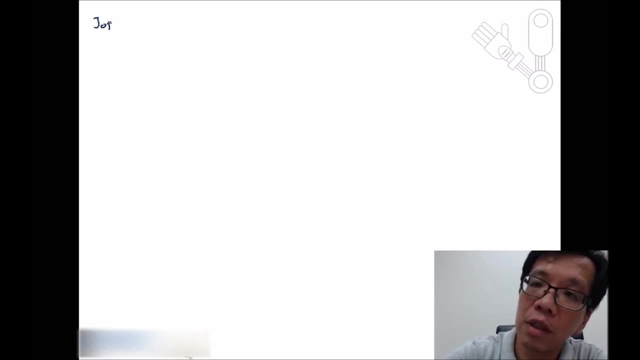 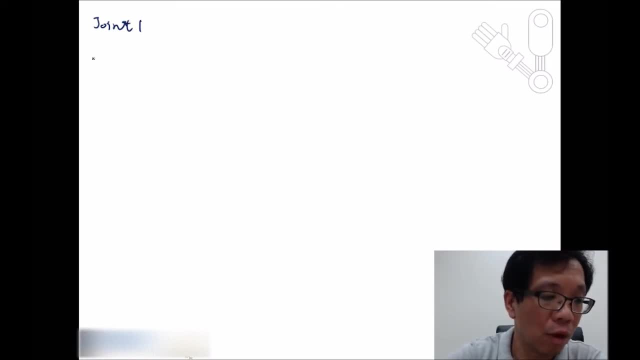 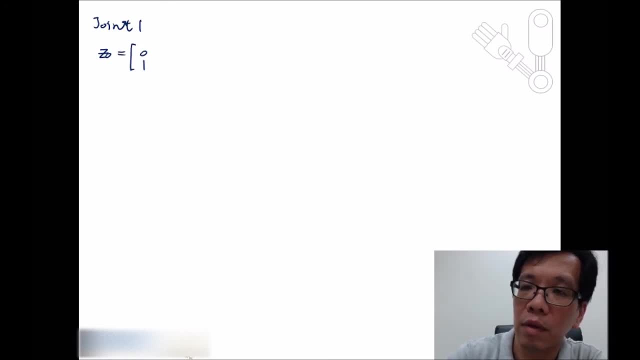 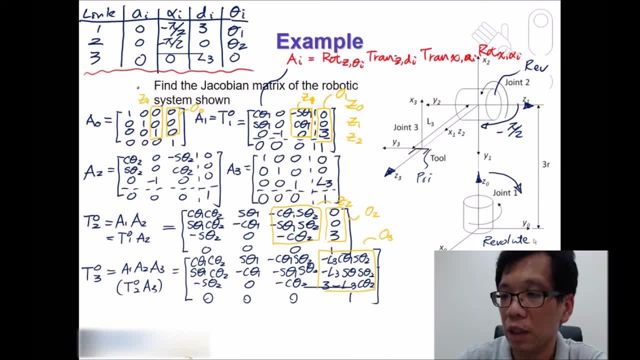 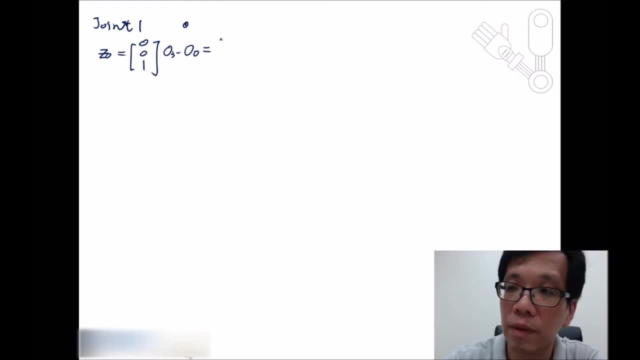 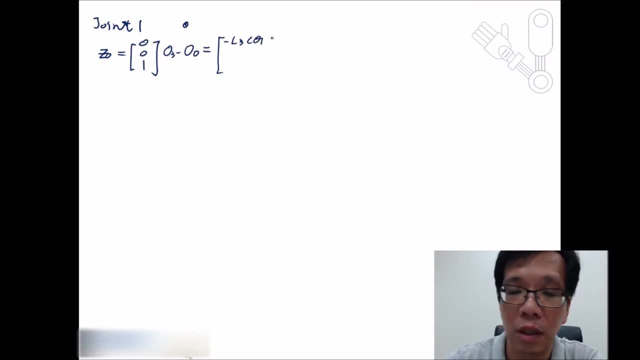 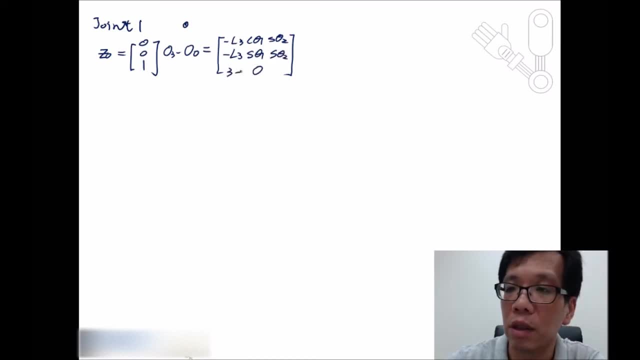 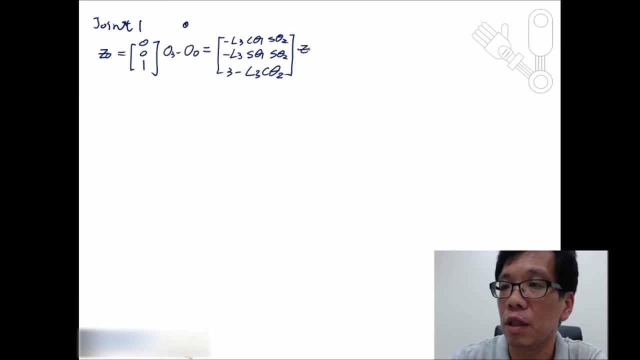 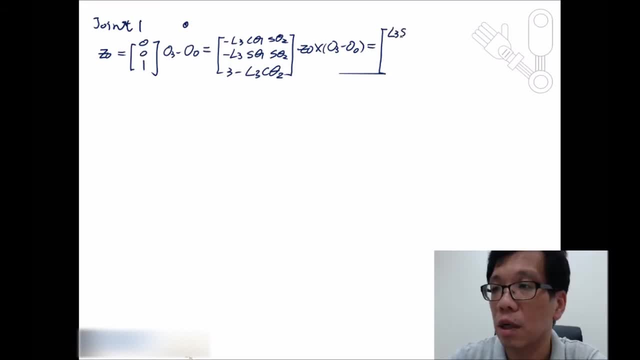 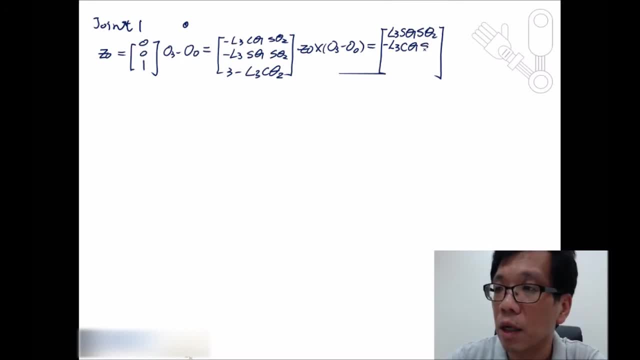 sine theta 2 and this component over here is 0. That is my JV1.. If you put those three components over here and put 0,, 0,, 1 over here, that is your J1.. Pretty straightforward For joint 2, still revolved. 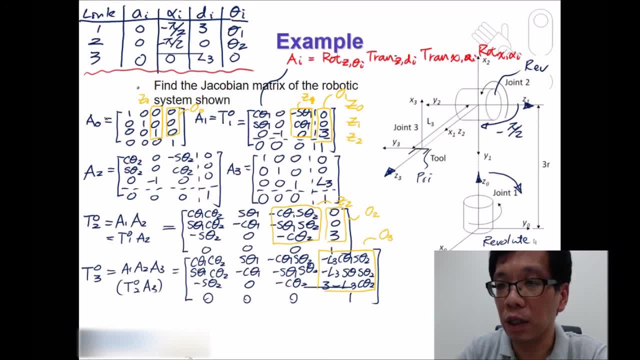 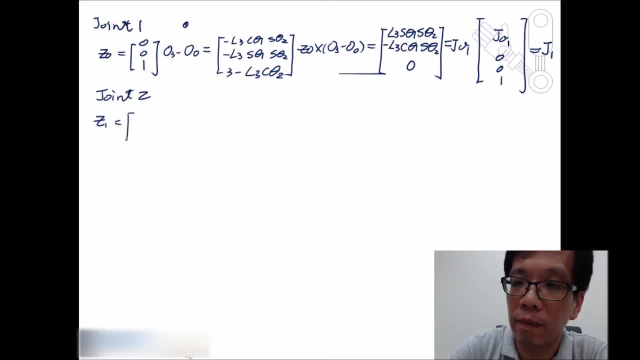 So you need to come up with Z1.. Z1 in this case is going to be negative sine theta 1 and cosine theta 1.. The third column over here is 0.. 0, 3 minus 0, 1.. 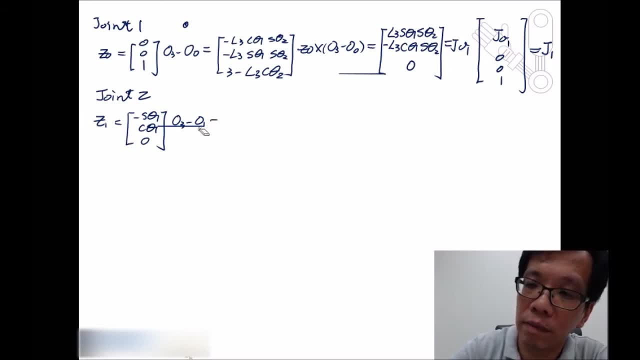 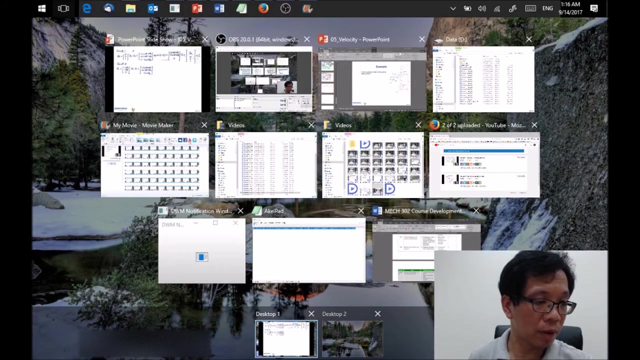 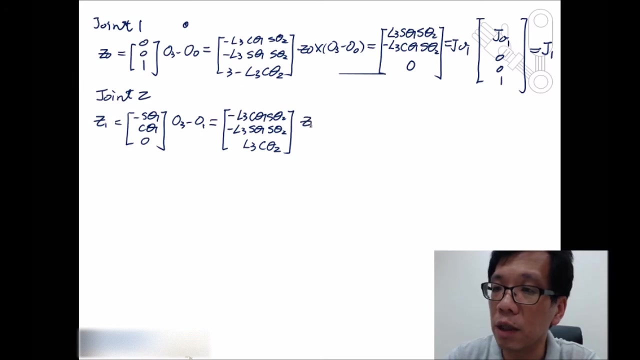 0, 3 minus 0, 1.. 0, 3 minus 0, 1.. equals to this one. Ok, So when we are doing this one, our Z1 cross product, O3 minus O1, that will give us negative L3. cosine theta 1, cosine theta 2,. 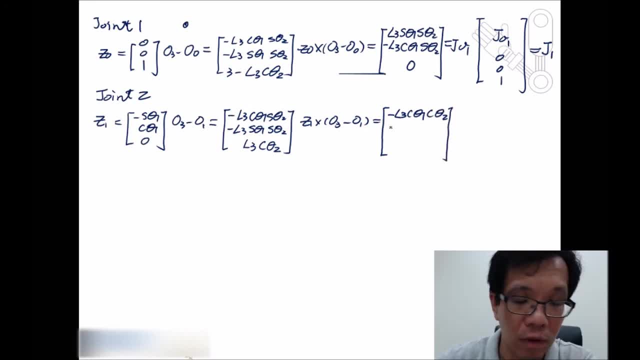 negative: L3 sine theta 1, cosine theta 2, L3 sine theta 2, that is my JV2.. And J2 is going to be JV2.. Over here it's going to be negative sine theta 1, cosine theta 1, and 0, which comes from here. 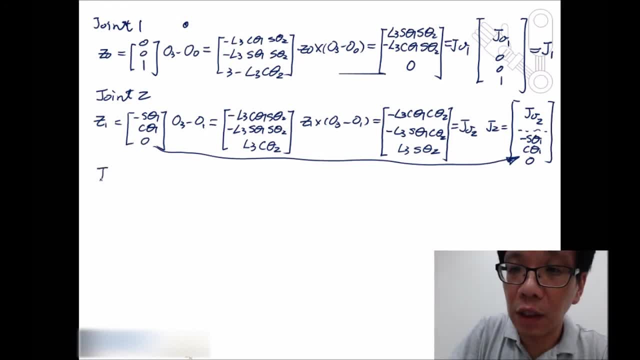 Okay, so that's my J2.. For joint 3,, this time it only includes linear movement And if you check back to what we have, we got my Z2 equals to negative cosine theta 1, sine theta 2,. 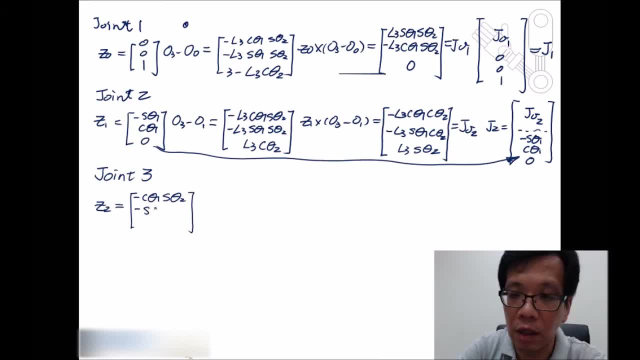 negative sine theta 1, sine theta 2, negative cosine theta 2, which is this one over here. Now, keep in mind, this one over here is prismatic, So the formula we're going to use is going to be a little bit different. 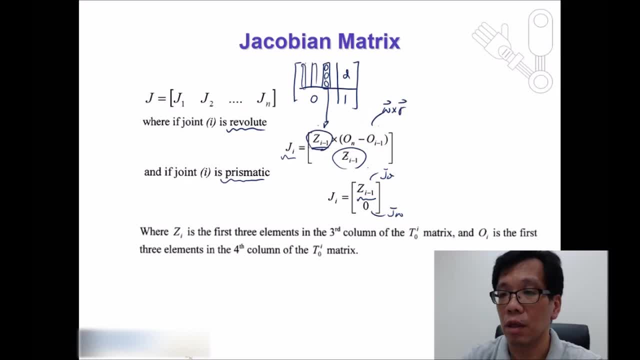 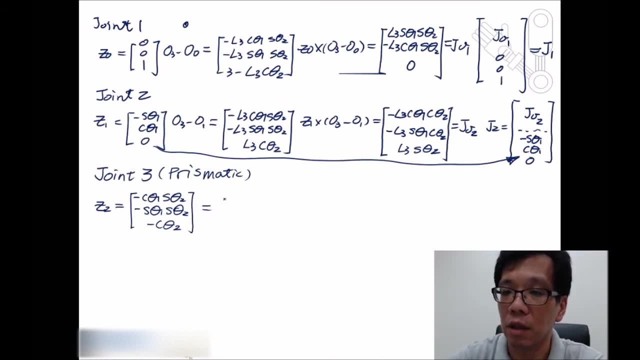 which should be. let's move back to this. It should be this one. So this is going to be Z2, and the rest of three components is going to be 0.. So we're going to be going to be 0.. 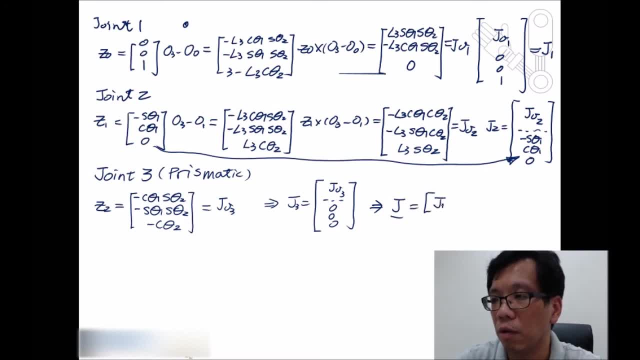 Okay, So we're going to take this, this promised molecule, over here. the injury line: 0 and 0, inside 0.. So we're going to take this, this hosted formula, all over here: 0.. J equals to J1,, J2, and J3.. 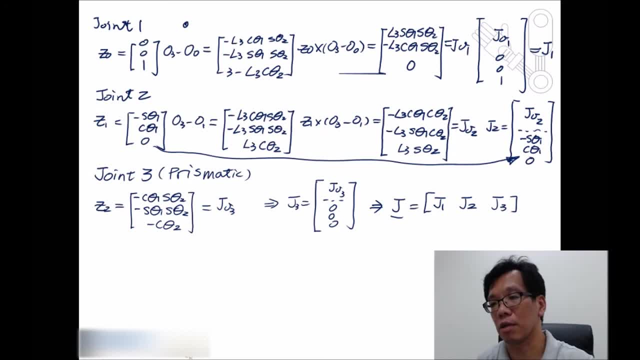 If you put all the components all together, they will be synthesized into this specific Jacobian matrix And that is something we're going to use for calculating other stuff. So that's, if you just want to find out a Jacobian matrix, this would be the answer. 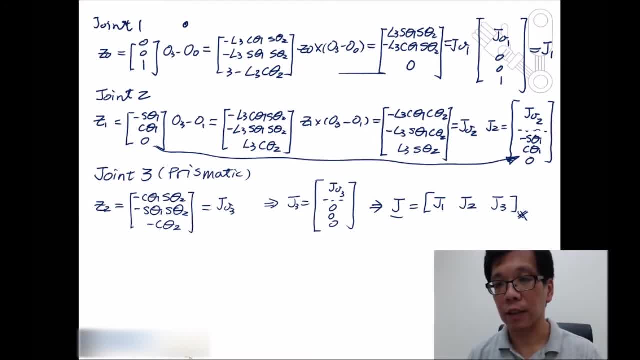 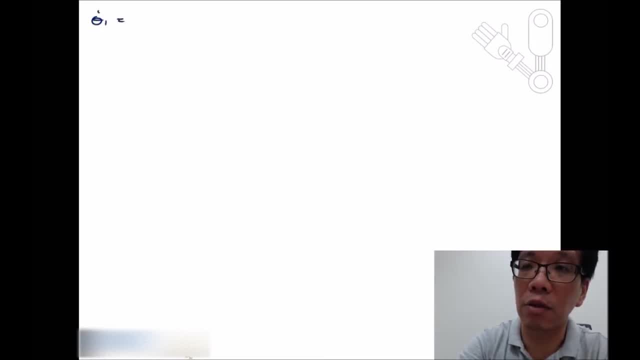 But let's do something. furthermore, Let's assume I got my theta1 dot equals to 2 radians per second, My theta2 dot equals to negative 1 radians per second And join 3.. My theta2 dot is locked at 2 meters. 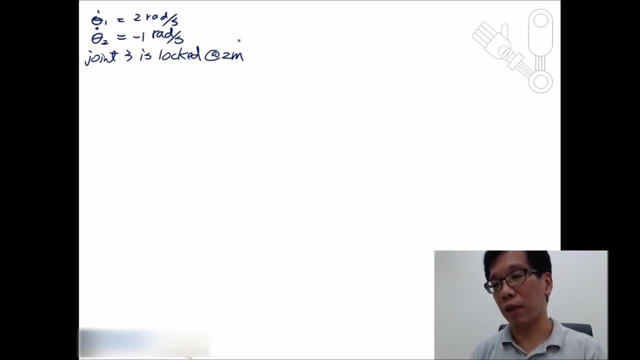 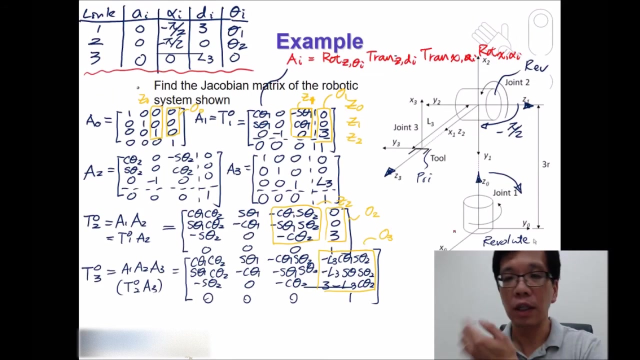 So when we come up with this specific configuration, what we need to do is to find out: what are we actually dealing with right now? So let's do this. OK, Let's go back and check the configuration over here, because this time we do need to. 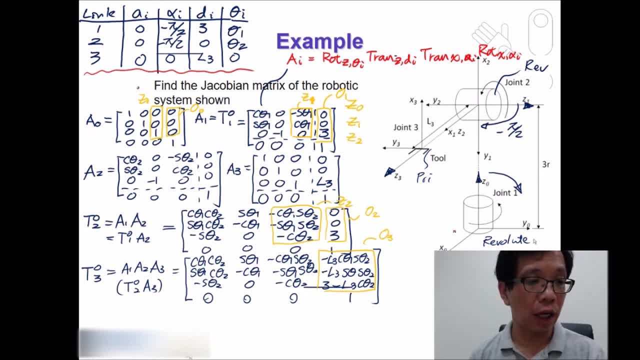 know what is my theta1,, theta2, and the information we have at L3.. So, before we move on, my theta1 in this case equals to 0 degree and my alpha equals to negative 90 degree. My theta2 equals to minus 90 degree. 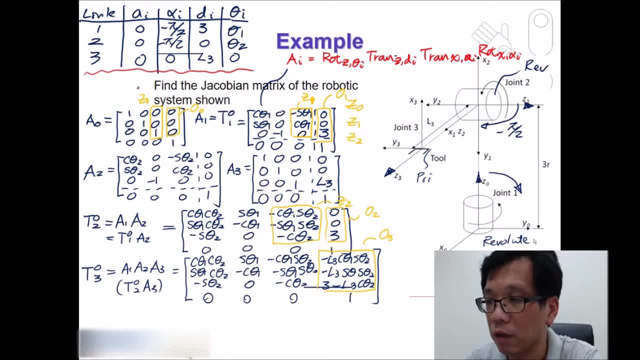 And my alpha2 is going to be negative 90 degree. So we adopt this one and this one over here. That is because the angle is not going to be changed, But over here we've got theta1 and theta2.. They are variables, not 0 degree and negative 90 degree. 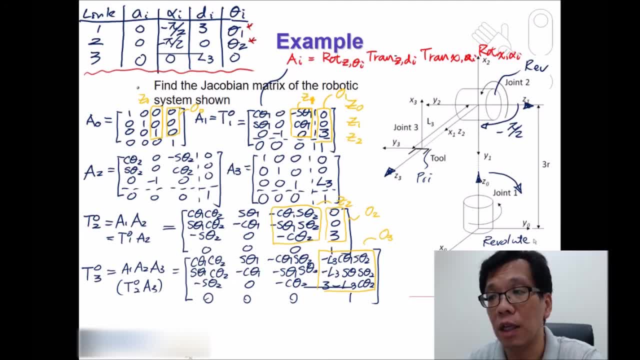 That is because it is always rotating and we need them to be variable. But when we try to come up with the information of velocity, we cannot have them as a variable. We need to know at this location what is my current angular velocity and what is my position. 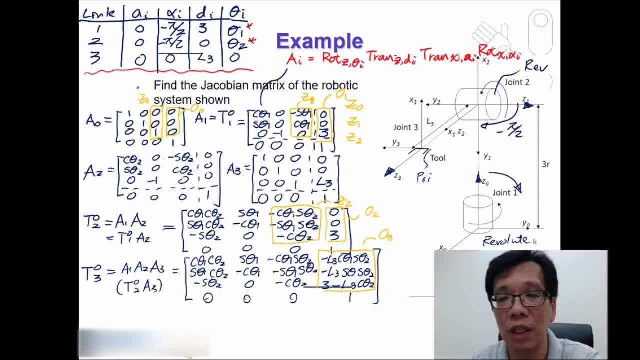 Then I can start to solve for everything. So, based on this configuration over here, theta1 equals to 0 degree and theta2 equals to negative 90 degree. And also, in this case, my L3 is being locked at 2 meter, which means the velocity is going. 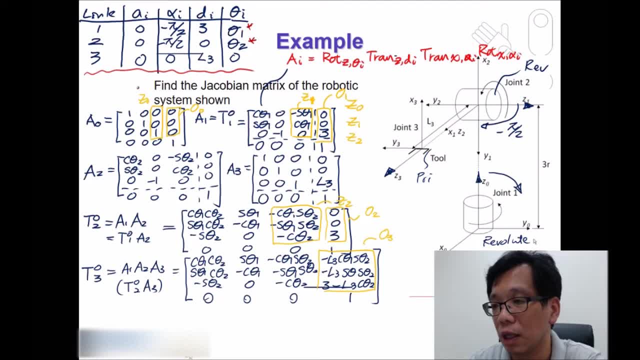 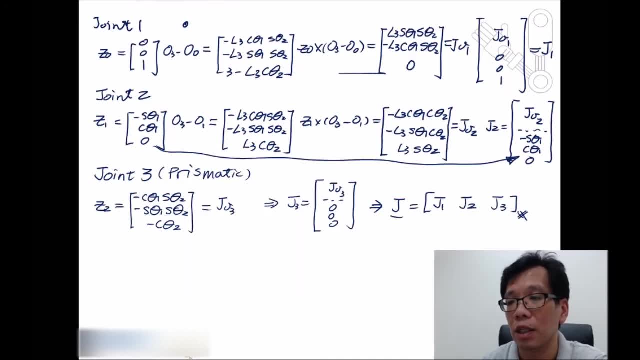 to be 0 for that specific joint. So with those information we can start to come up with the answers. One of the most important thing we need to do is to come up with- Let's do it over here- Jb and j omega. 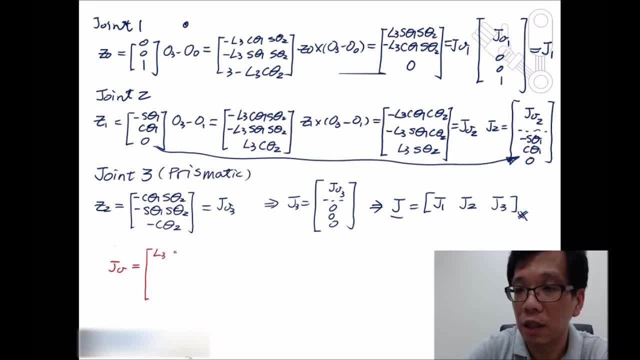 Jb over here is going to be L3, sine theta1, sine theta2, negative L3, cosine theta1, sine theta2, and 0.. For the second column over here, it's going to be this: 3 column. 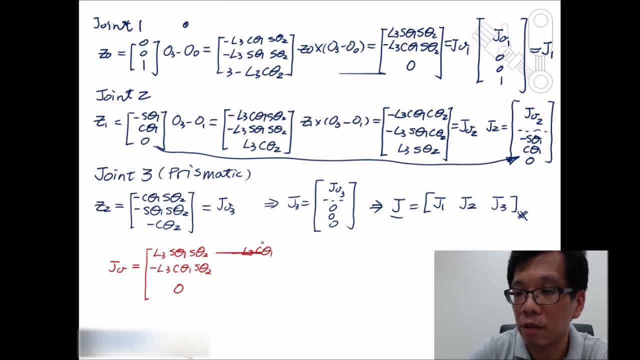 Again, we'll be�. For the second column. we need to add these 3 components: sine theta1, cosine theta2, L3, sine theta2, and over here I got negative cosine theta1, sine theta2, negative sine theta 1, sine theta 2,. 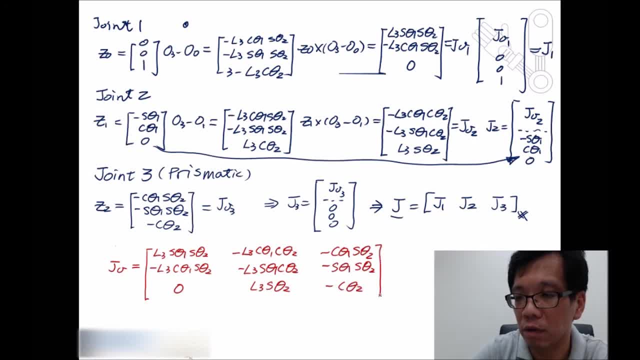 negative cosine theta 2, that's my Jv for my j omega 0, 0, 1.. Second one over here that is going to be negative sine theta 1, cosine theta 1 and 0. And over here I got 0, 0. 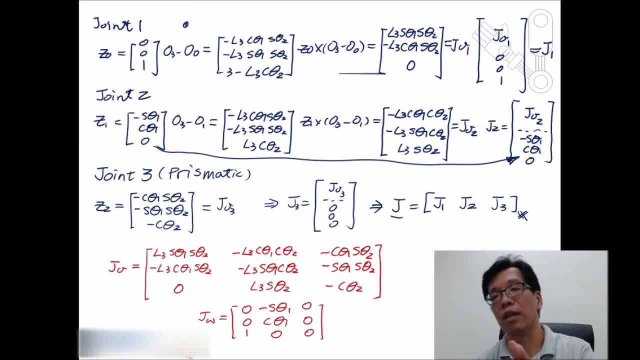 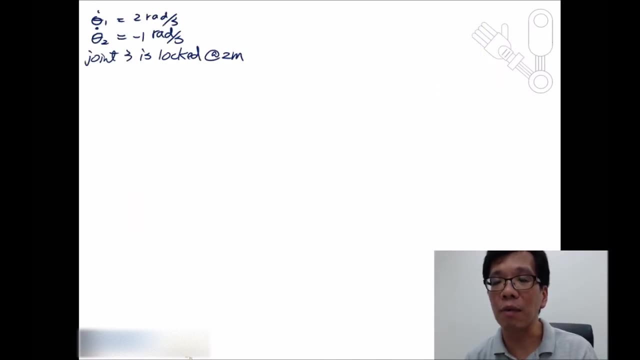 and 0. So if you combine again, if you combine those two together, that is going to be your J matrix, This one and this one. But since we are not trying to find out a Jacobian matrix, this time we want to find out. 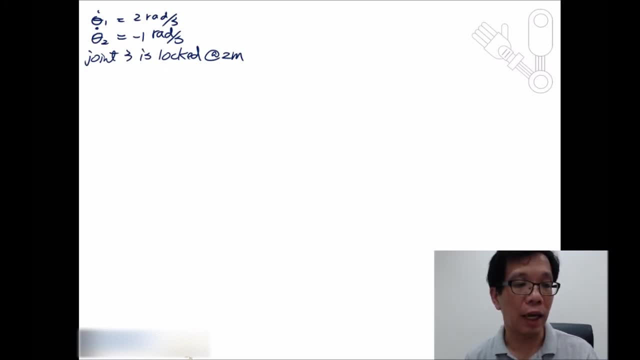 what is my velocity and what is my, my, Q, those kind of information. So what we're going to do is to generate Jv with theta 1 equals to 0 degree, theta 2 equals to negative 90 degree and l3 equals to 2n. 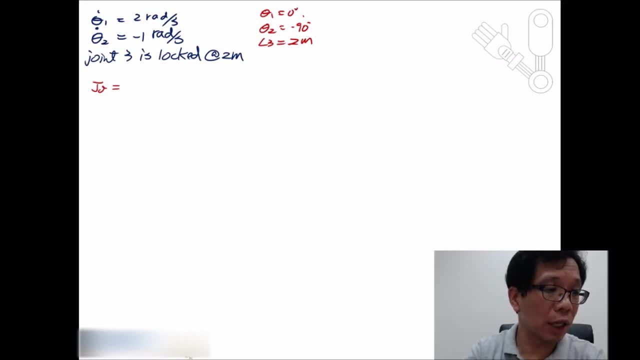 So if we get everything all together, we are having my Jv equals to 0, 2, 0, 0, 0, negative 2. 1, 0, 0.. j: omega 2, 0, 0, 0, 0. 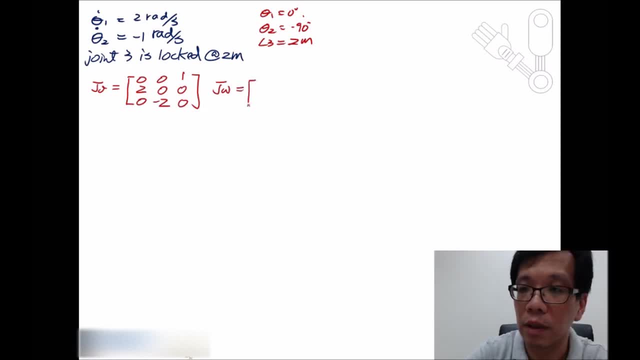 is going to be 0 0 0, 1 0, 1 0 0 0 0.. So again, if you want to find out all six components, all six velocities, you can just combine JV and J omega together to 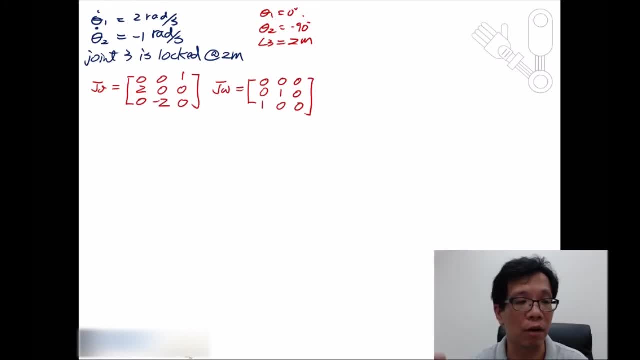 synthesize a big J matrix. But if you just want to find out the information of linear velocity, then, since we are talking about linear velocity, what we're trying to get is the matrix of JV. So what we're going to do is to use JV. 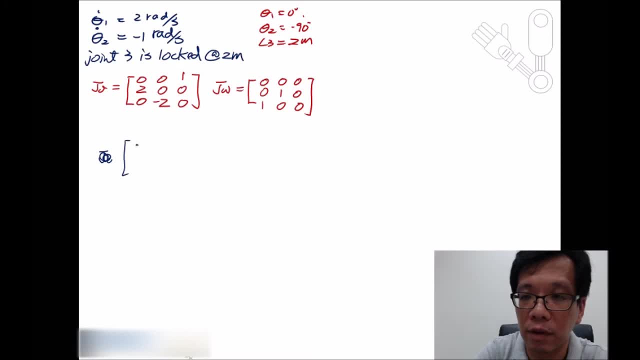 x dot, y dot, z, dot equals to vx, vy z. That is going to be JV multiplied by zeta 1, dot, zeta 2, dot and v3.. This one over here, v3, equals to 0, because it's. 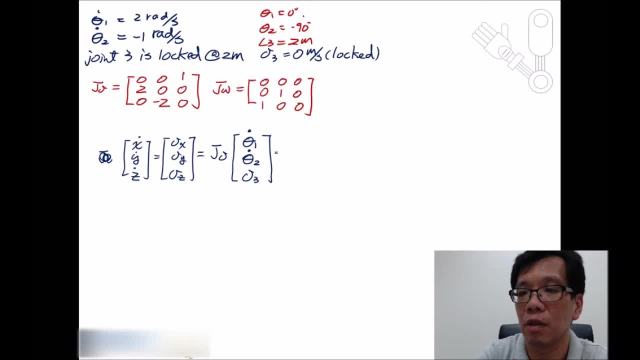 locked. So it is going to be 0, 2, 0, 0, 0 negative 2, 1, 0, 0, 2 negative, 1, 0.. In this case you're going to identify this is going to be 0, 4, 2 meter per second. That is how we use. 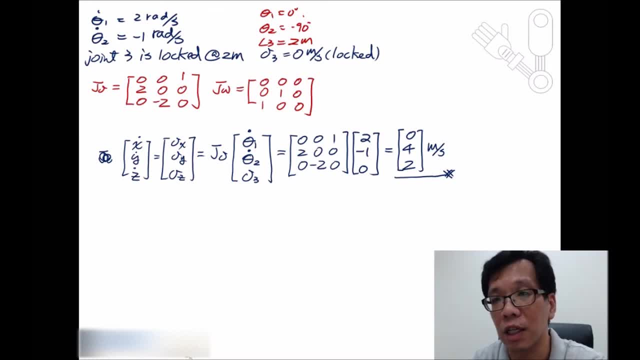 Jacobian matrix To come up with the velocity based on the information, or the angular velocity, linear velocity of each joint measured locally. Okay, this is going to be important for us because with those information it's more convenient for us to come up with all the information, with all the matrix information, and we can.